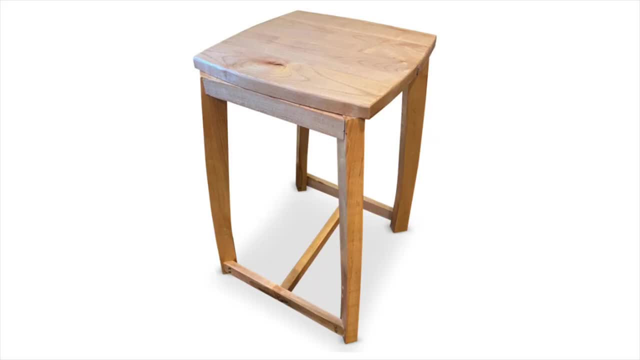 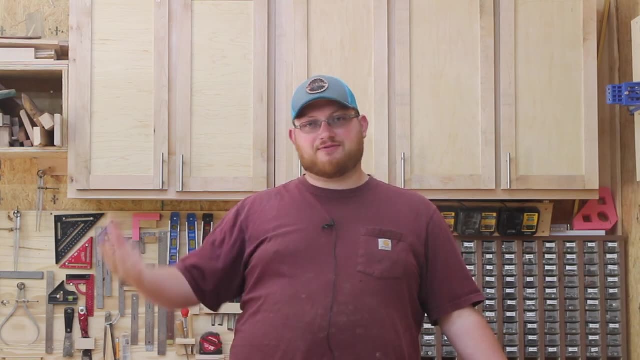 pocket holes or butt joints and wood glue, things like that. You don't have to make a curved seat. You don't have to make a curved back support. You don't have to make curved legs. That's all more advanced stuff. But the reason why a stool is such a good starter project is for that reason. 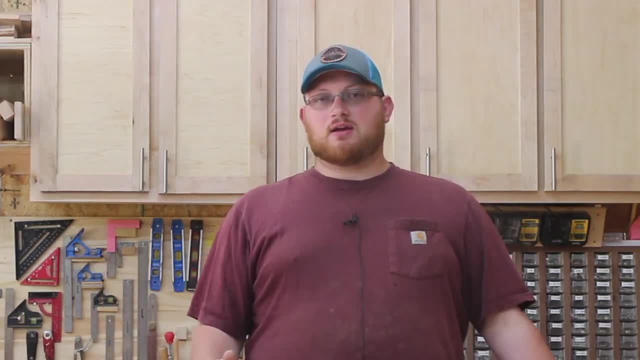 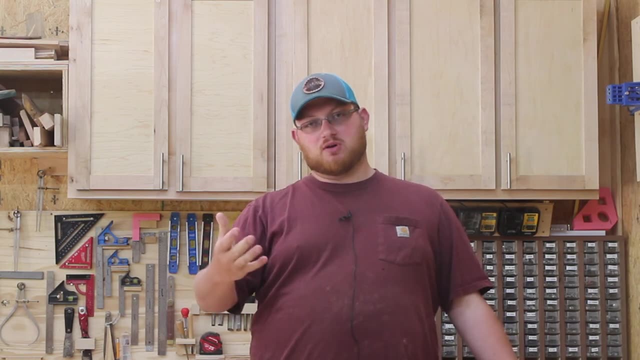 It can be as basic or as elaborate as you would like. Another good thing about using stools as a starter project is that they're relatively quick. A lot of stools can be made, start to finish, in just one day, which will help keep you motivated. These stools can also be made. 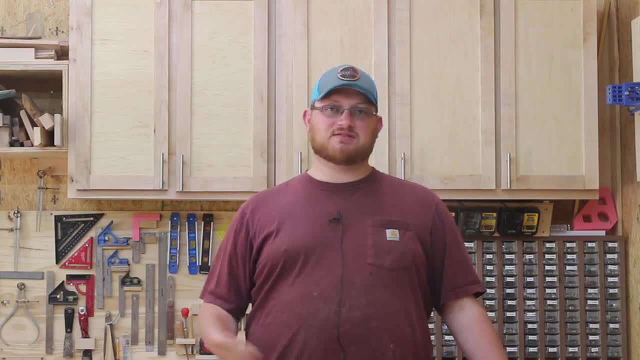 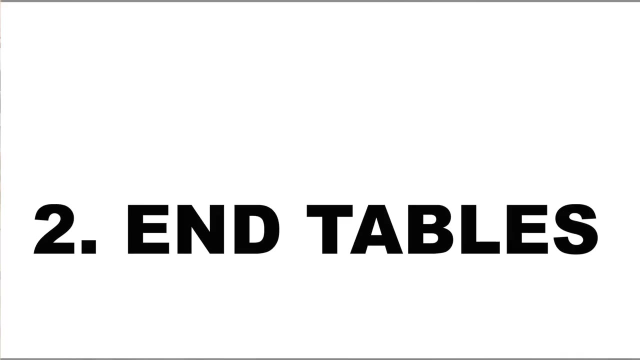 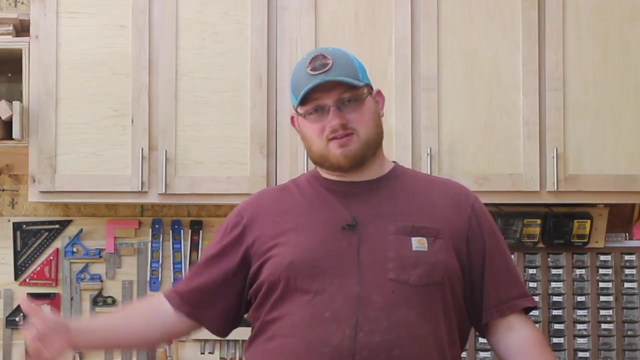 from cheaper lumber, cheaper materials, Sometimes even building materials, so that you're not investing a huge financial investment in your project. So if you mess up, you're not losing that much. Project number two is end tables. Now, when I say end tables, I mean like nightstands, coffee tables, end tables on the end of your couch. 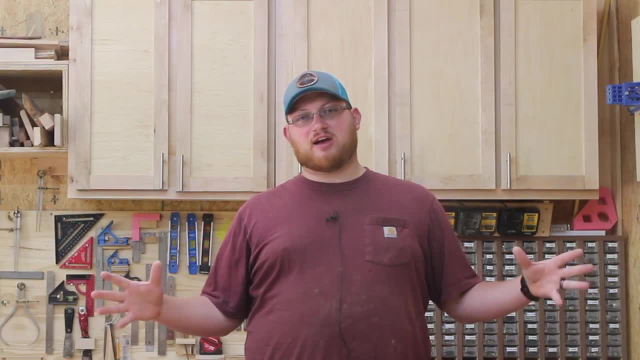 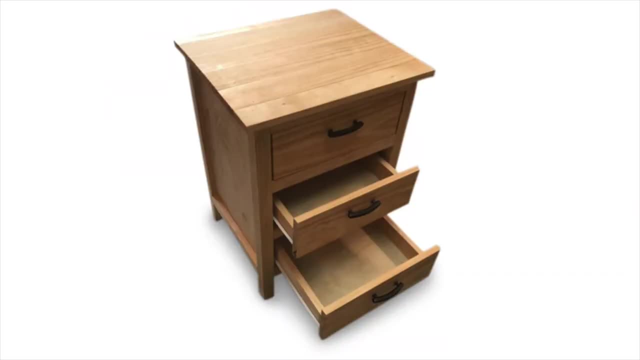 a true end table whatever, And the reason is because these are so vast in the style, design, size, etc. The good thing about end tables is they can be again as basic or as elaborate as you would like. Some end tables just have some legs and a top. 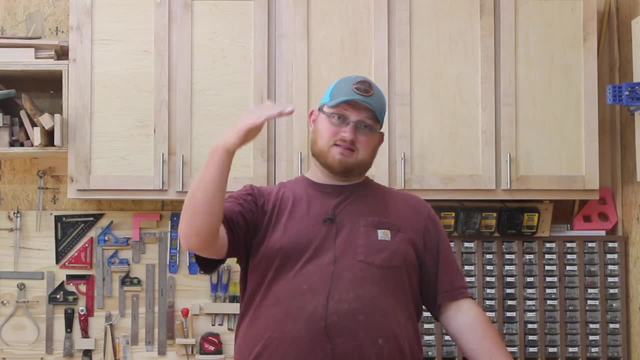 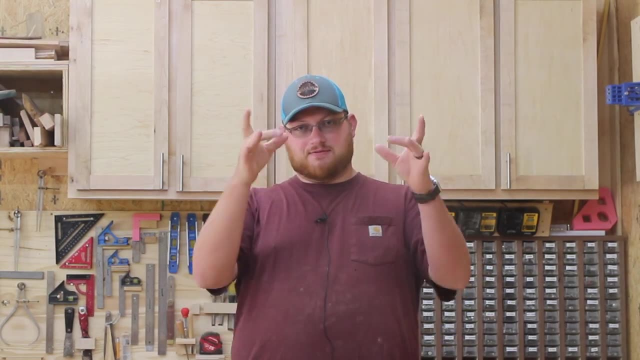 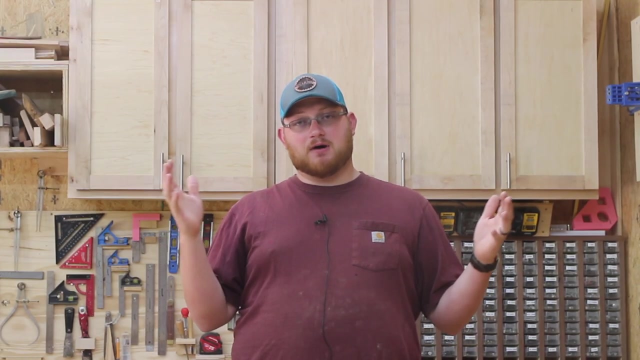 Some have legs, a top and a shelf. Some have a top legs, shelf and drawers. Again, you can make it as elaborate as you would like. You can start with four basic legs of square posts with a tabletop and maybe one shelf. You can move up into adding fancy drawers. You can do dovetails on those. 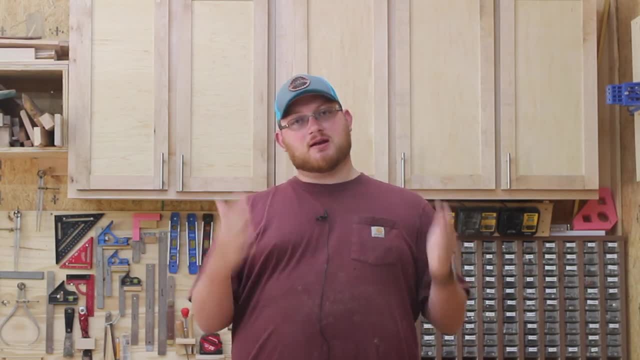 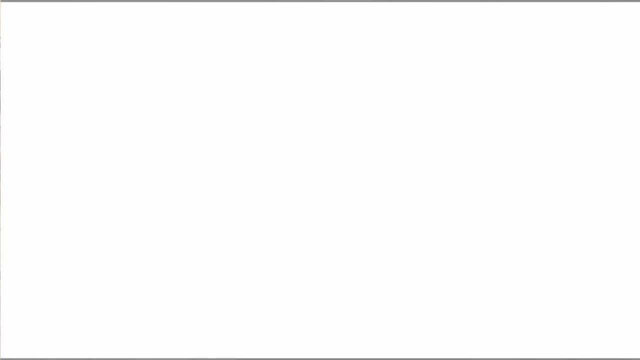 drawers. You can do anything you would like as you grow your skill set, But an end table is a really good place to start as well. The third project for beginner woodworkers are boxes. Now, boxes, again, can vary. What I'm talking about are small boxes, And the reason this is a good project is because 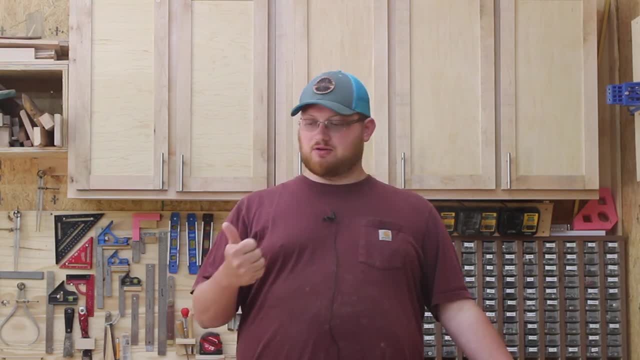 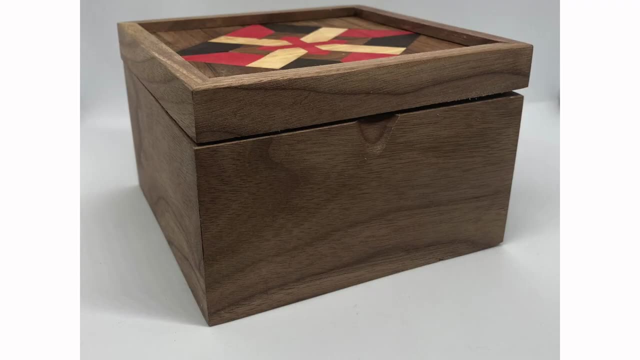 it allows you to practice different styles of corner joinery. You have miter joints, box joints, dovetail joints, mortise and tenons, And those joinery methods can be as elaborate or as simple as you would like. A lot of small boxes start with just wood glue. Then you might move up to wood glue. 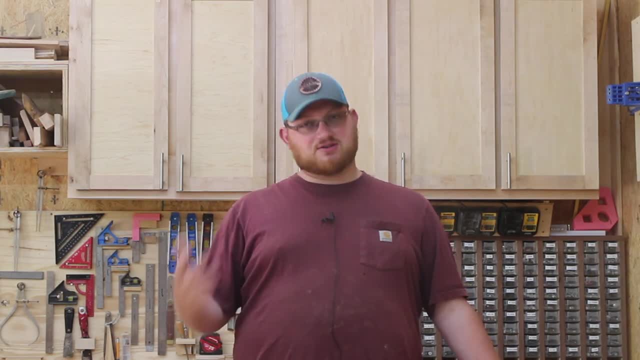 and a dowel joint or a box joint or a dovetail joint as you grow your skill set. The good thing about boxes as well is a lot of the times they're small enough where they can be used with very little effort. Some even use scrap wood And scrap wood and small cut-offs, small amounts of material. 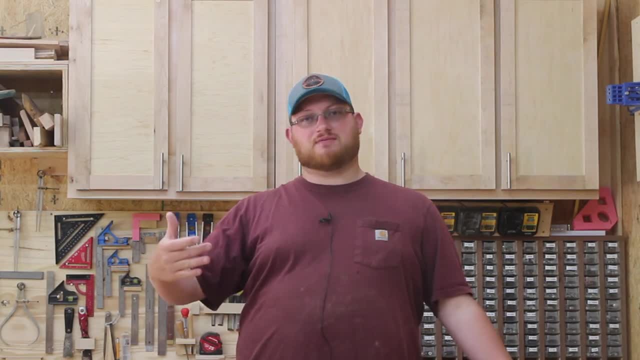 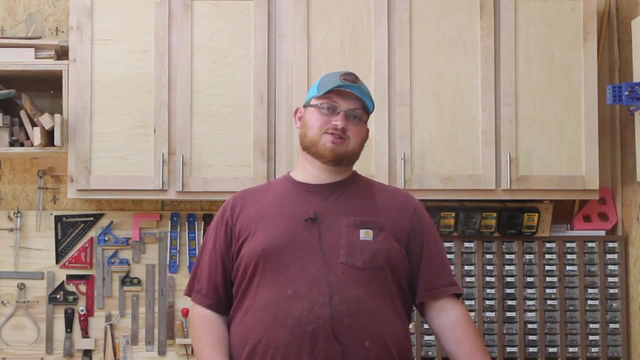 again, are cheap, easy to get your hands on, So you're not putting a huge financial investment in up front. So if you do mess up while you're learning, you're not spending a whole lot of money. The second reason why a box is a good starter project is for trims and molding Some boxes. 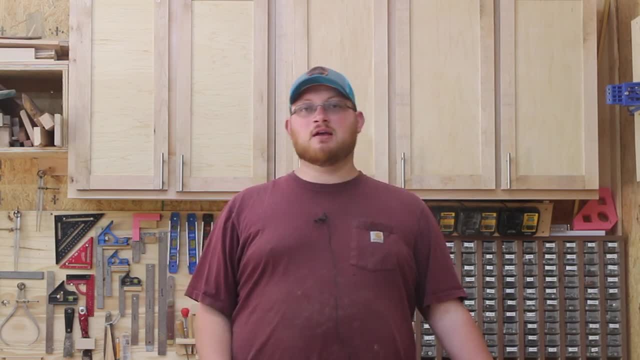 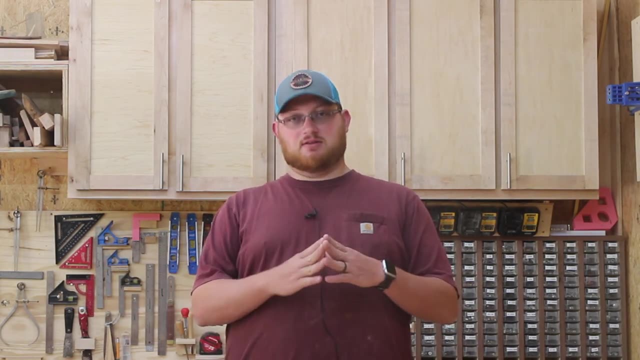 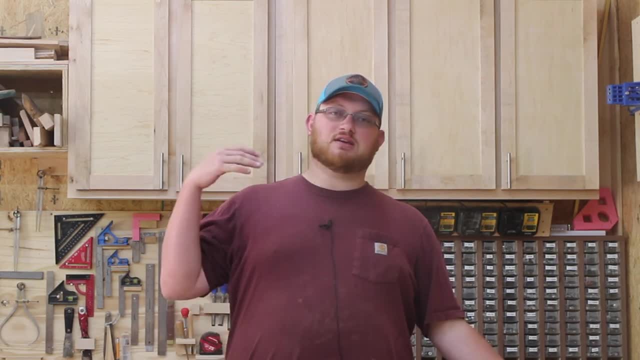 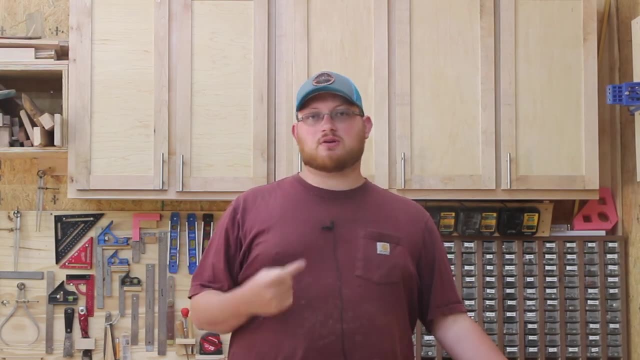 Another good reason for practicing with boxes is that it allows you to get accustomed and acclimated to how your wood and your species of wood that you're using on your box reacts when you're machining it, Using your jointer, using your saws. It allows you to get a good grasp on. 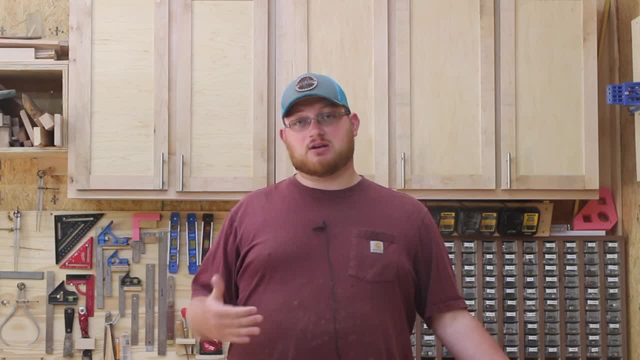 how that wood is going to react and how well or not so well it's going to machine with that. tool Boxes are also good for starters because they make great gifts. A box can pretty much be used for anything. It can be used as a keepsake or a memento box. It can also be used as a 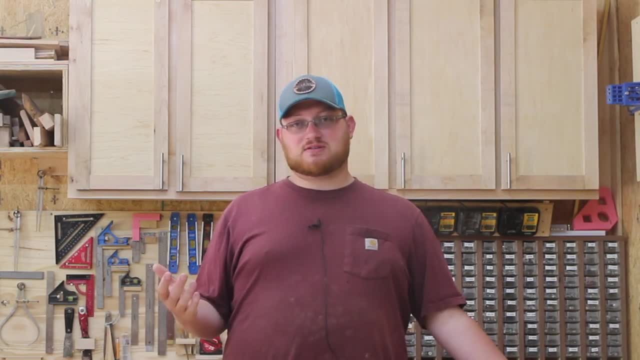 box, a valet tray, a valet box. It can also just be used for a practical reason, A pencil box or a keychain box or a collection box, coin box, And these boxes are usually small enough to where, if you practice and you make 10 of them, you're not using up a lot of storage space to keep them You. 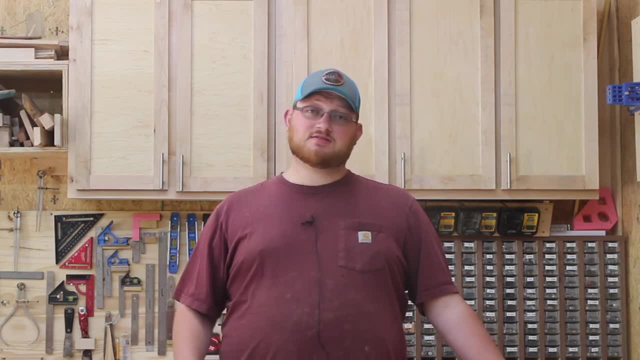 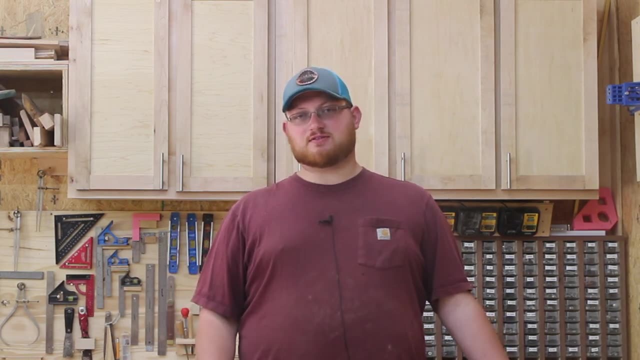 can put them all in one area and keep them relatively easily. That also goes for the boxes that you gift to other people. They're an easy gift because they're easy to store. They don't take up a lot of space. The fourth starter project is a cutting board. Now, when I say cutting board, 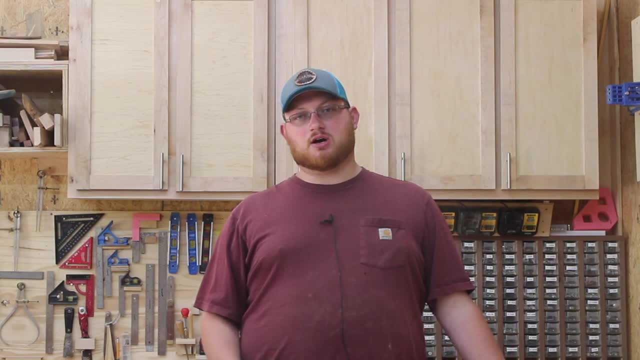 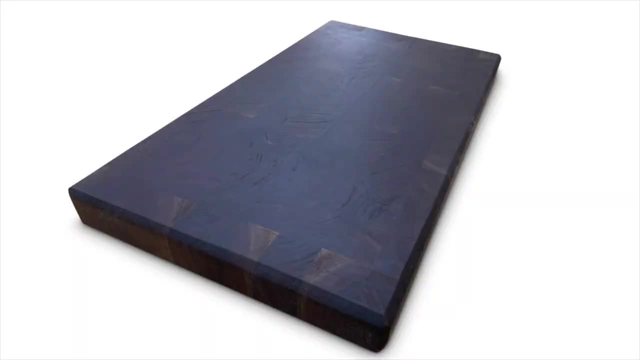 I'm talking about a solid piece of wood that you make into a cutting board. If you're doing a cutting board, that requires a glue up with long grain or edge grain, that's a little bit more elaborate because there's more milling and more gluing and more processes involved. But if you do, 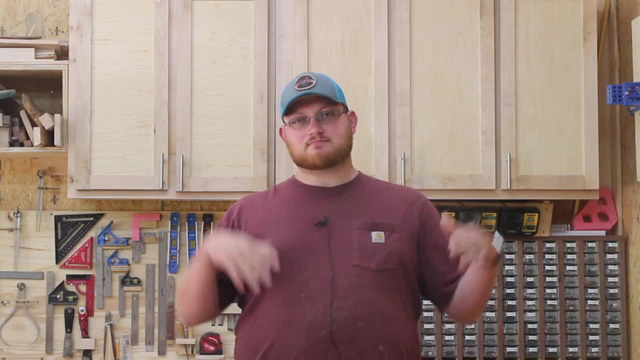 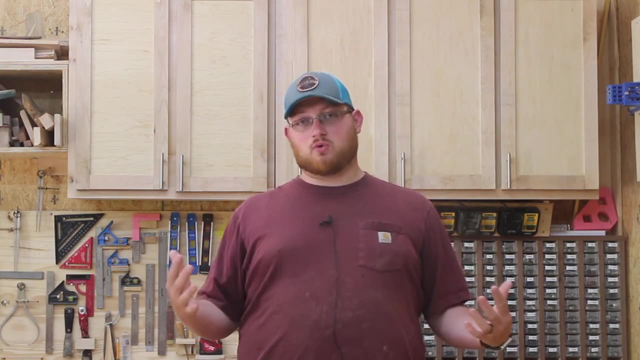 a charcuterie style board where it's just one solid piece of wood. this is a good starter project to get you accustomed to milling the wood, getting it flat and square. It also introduces you slowly to rounded corners. You can make a rounded handle. You can make a juice groove, You can make a rounded. 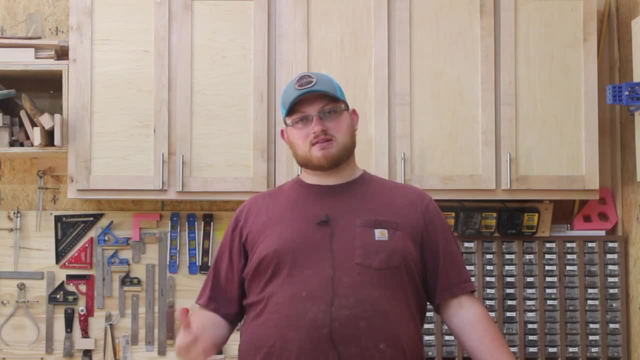 corner, on all the sides of the board, et cetera. It's a good way to start and a good way to get used to working with wood. The fifth and final starter woodworking project that I recommend are shelves and bookcases. I recommend shelves and bookcases simply because it introduces you slowly to making larger scale.